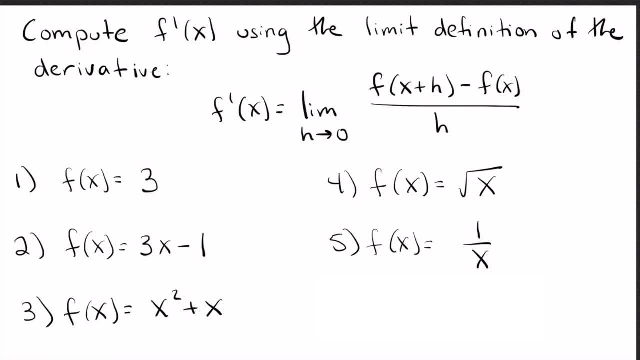 So in this video we'll be working through a bunch of problems taking the derivative, using the limit definition of the derivative. If you want, you can just skip to exactly the kind of problems that you feel are most appropriate for you. So these problems really take you from just. 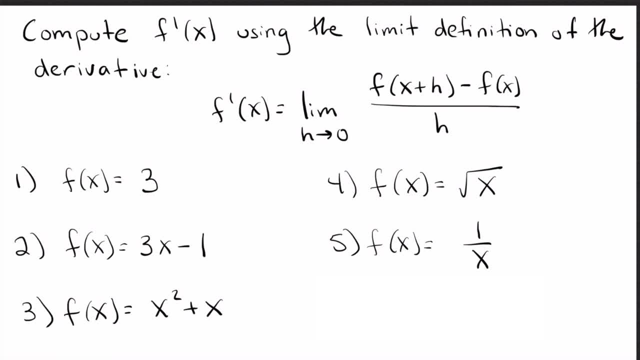 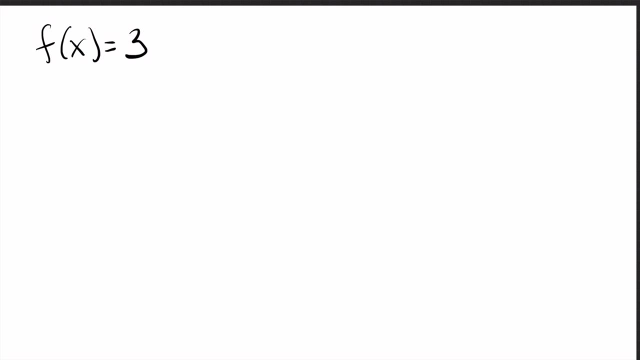 about the easiest type of limit derivatives you can take to just about as complicated as you can go, And with the skills from these you can do most basic problems of this type. So let's go ahead and get started with number one. So the first one is just taking the derivative of a. 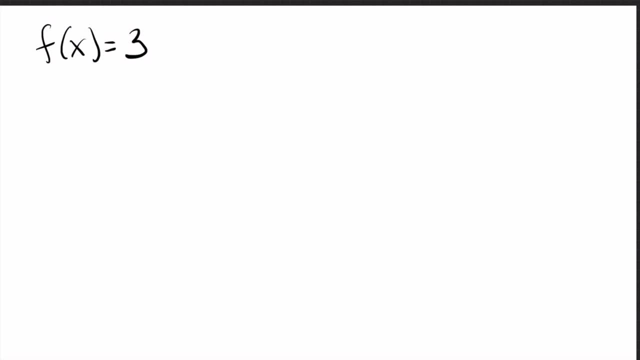 constant of a number. There's nothing special about three. This works exactly the same for zero or negative, 12 or pi or whatever. So let's go ahead and get started. So remember that the derivative of f is given by the limit as h goes to zero. So this is what we refer to as the limit. 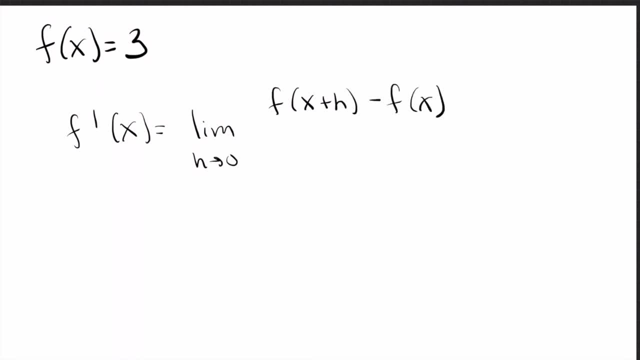 definition of the derivative. So for this one we'll really focus on understanding what each part is And then the later problems. we'll just assume you understand that. So the first thing here is f of x plus h. So that means take the equation f and replace any x's you. 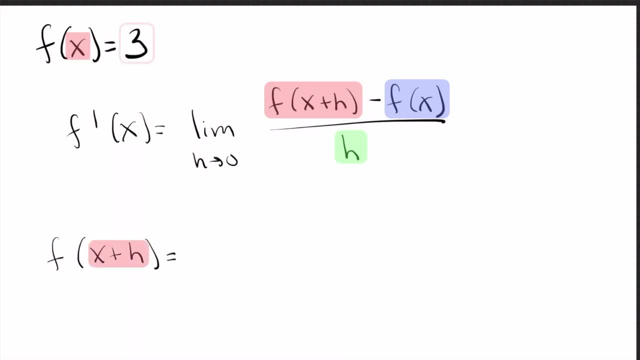 see, with an x plus h. Well, on the right there are no x's, right It's just a three. So there's nothing to replace, It just stays three. So that makes it pretty easy here. So let's go ahead and 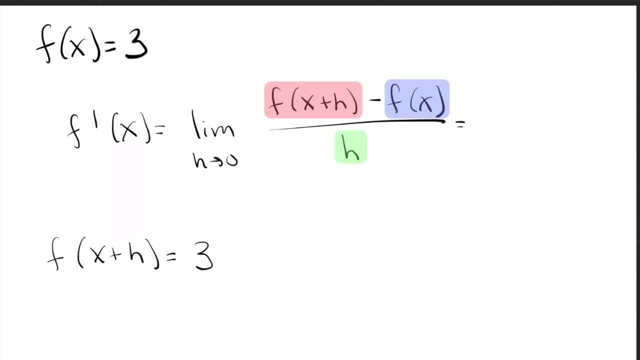 do that, So I'll go ahead and plug those in, And if I do that, what we see is f of x plus h is three. What is f of x? We just look up: top f of x equals three And on the bottom h is just h. 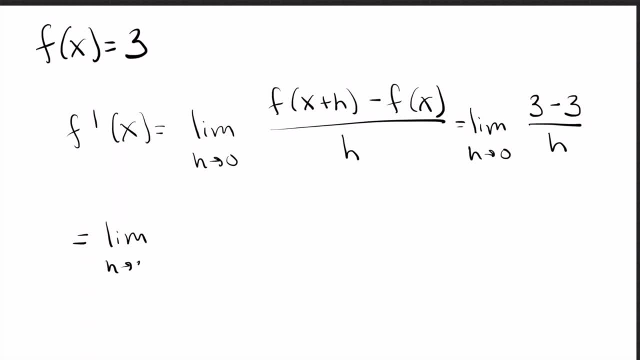 Okay, so of course that just becomes zero. on the top. We get zero over h. Zero divided by any number is zero, So that gives us zero, Okay. so one thing that I know some people struggle with is right here. Normally when you take limits, you want to plug. 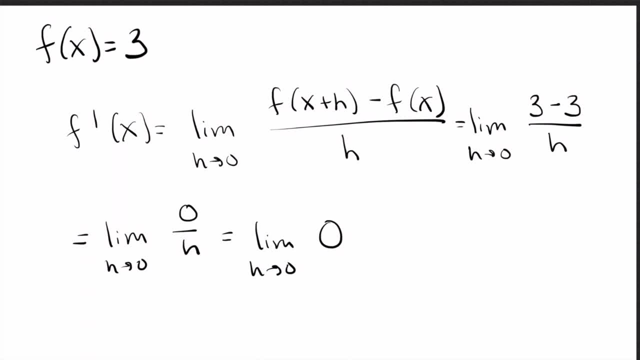 in h equals zero, since h is going to zero But there are no h's, So actually that means it's easier. So here I'm going to look at this and I'm going to change h to be zero. Well, there's no h's to change, So it just stays zero. So that is in fact the derivative of three. So here f, prime of x, equals zero. Okay, so let's go ahead and go on to the next one. 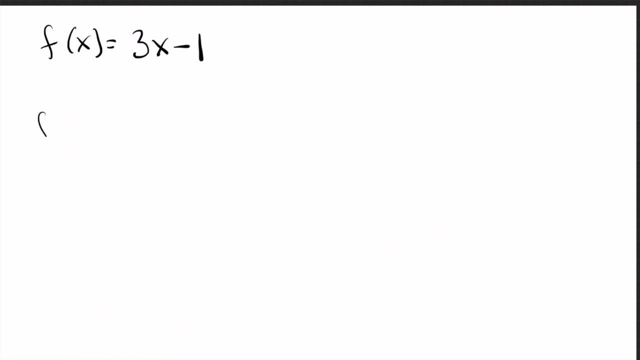 So now we're going on to sort of the next level up. So what we'll do is we'll start out exactly the same way. Just to help you out, let's go ahead and write out the whole limit definition of a derivative. So it's f of x plus h minus f of x over h. Okay, so let's compute on the side here: what is f of x? 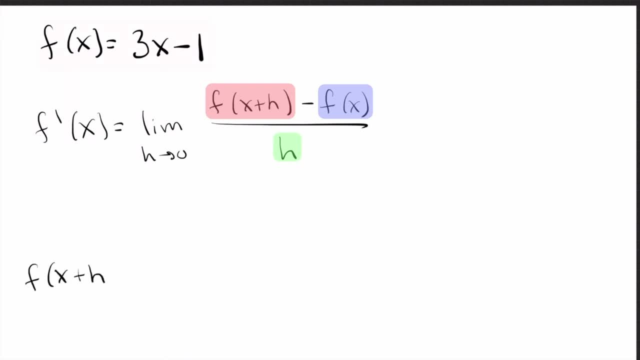 plus h. So f of x plus h means I take my equation any x I see, I replace it with x plus h And I You can generally do better if you put things in parentheses. You're less likely to make mistakes. Okay, so that's what f of x plus h is. 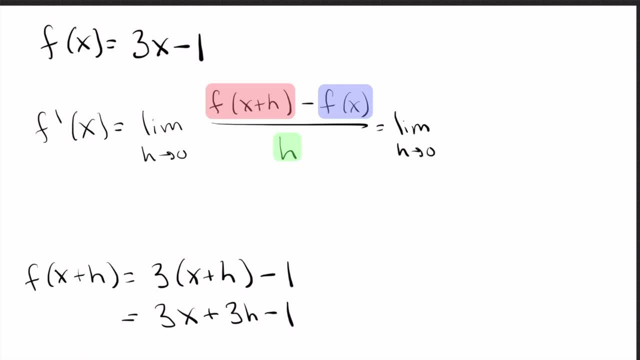 So let's go ahead up here and plug that in, So that becomes 3x plus 3h minus 1, minus f of x. What is f of x? It's 3x minus 1.. And our h on the bottom just stays h. 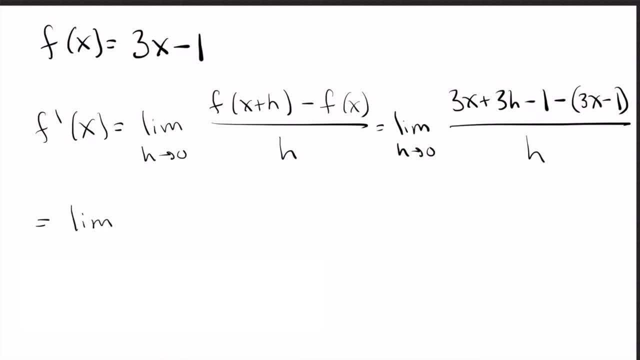 Okay, so the next step is really just to simplify this, to kind of clean it up. We've got some like terms on the top, So the first thing I'm going to do is just the negative in front of the parentheses here. I'm going to go and distribute that. 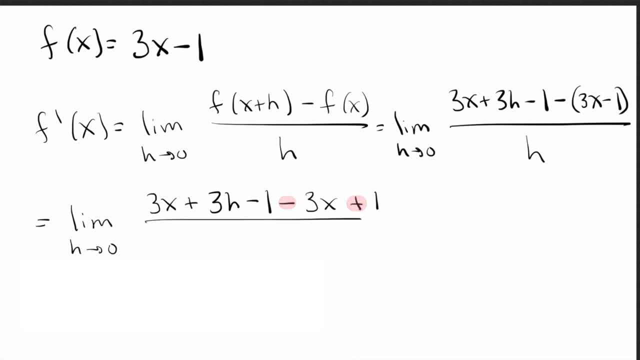 That gives me negative 3x and positive 1.. And next we've got some like terms, right. We can see that we've got on the top 3x minus 3x Those cancel out And we've got negative 1 plus 1.. 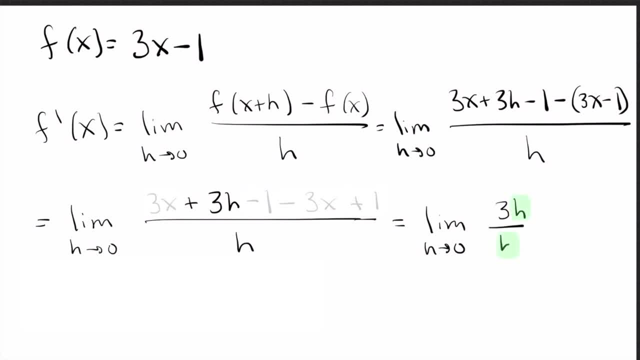 Those cancel out. So all we're left with is 3h over h, And so here the h's cancel, I get the limit, as h goes to 0 of 3. And this should look very familiar to the ones I did on the last problem. 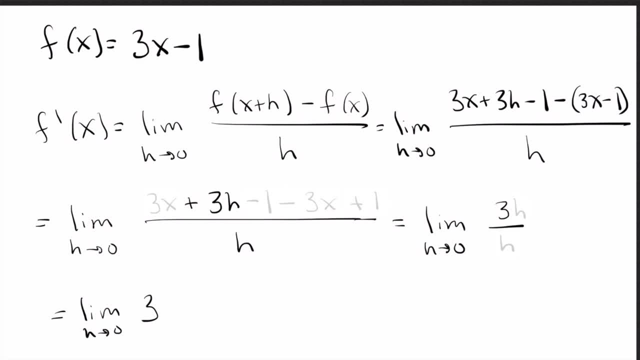 So we want to change h to be 0. Well, there's no h there to change, So it just stays 3.. So there we go. So to wrap it all up there, we get that the derivative of 3x minus 1 is 3.. 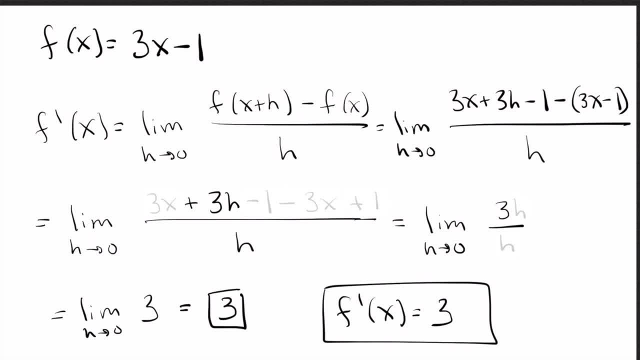 And there we go, Computed the second one. Okay, Let's go on, Let's go on to the third one. So here's where things start to get to be a little bit more work. It's not that they're necessarily harder. 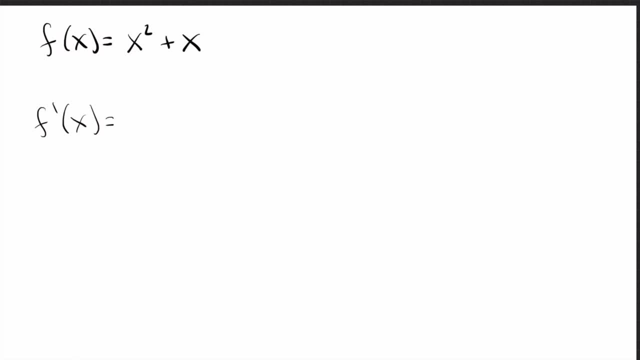 It's just that there's more steps involved. So at this point I'm going to go ahead and assume that I don't need to write the whole limit definition out. Let's just go ahead and do it. So I take f of x plus h. 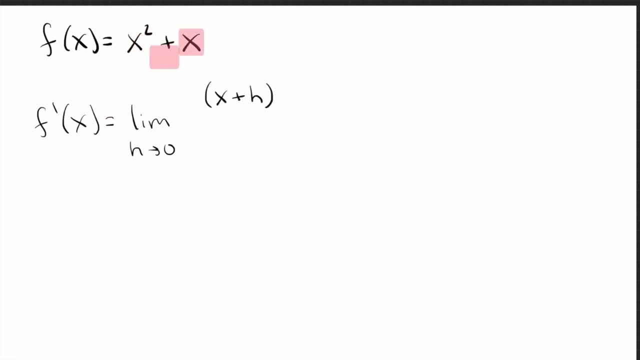 So I take my equation. I change any x's to be x plus h's. So that's what f of x plus h looks like, Minus f of x. Again, if you put this Things in parentheses, you're less likely to make mistakes. 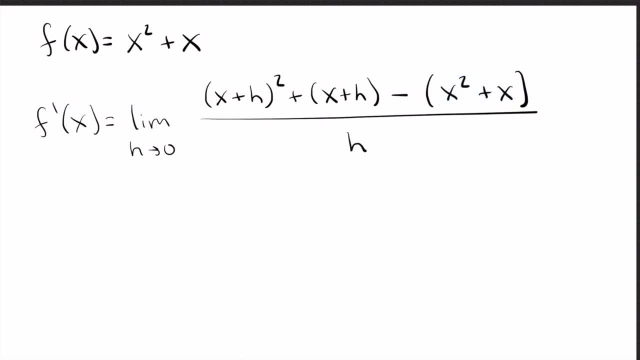 And I leave my h on bottom. So again here, what we want is to start simplifying and collecting like terms. So a common trick that shows up a lot is: if you've got something that you can square, often you should square it. 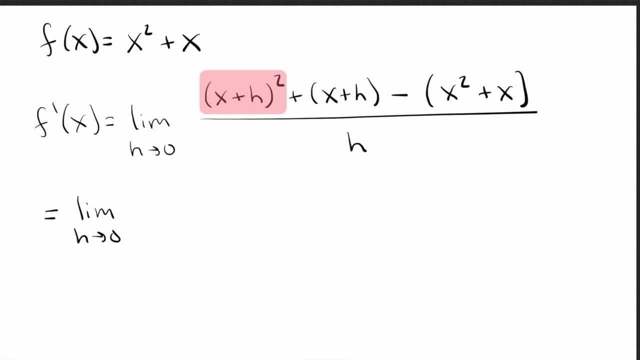 So up here I've got x plus h squared. If I do that, if I foil it all out, I get x squared plus 2xh plus h squared. Okay, So let's go ahead and just keep the rest of the terms. 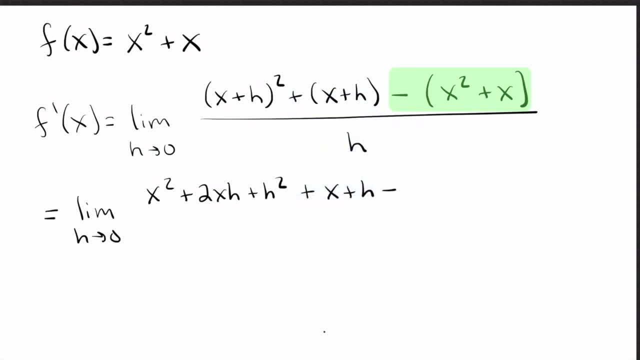 And while we're at it, I'm going to go ahead and distribute that minus sign So that becomes minus x, squared minus x. Now this might not be very fun, because you've got so much stuff all over the place It might feel like gosh, this is just getting horrible. 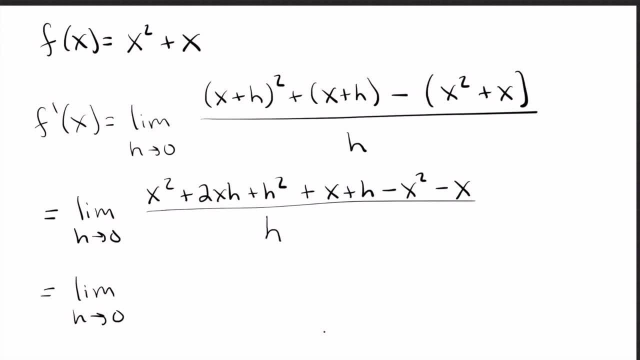 But the point is, as soon as you write it like that, you'll see that lots of things can cancel out. So I see I've got an x squared and a minus x squared. Those cancel out. I've still got my 2xh here. 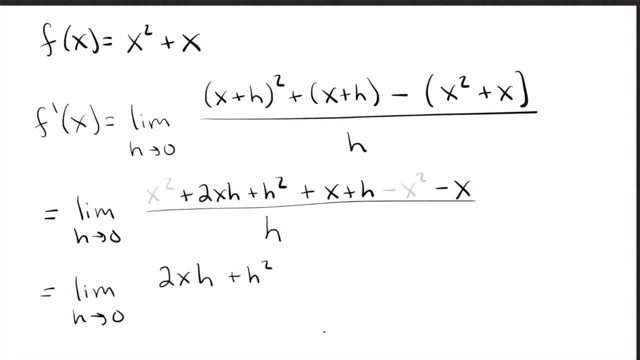 So let's go ahead and leave that. I've still got my h squared. Let's leave that. Then I've got an x minus x Those cancel out. So all I'm left with at the top now is that h. Then, on the bottom, I'll leave my h. 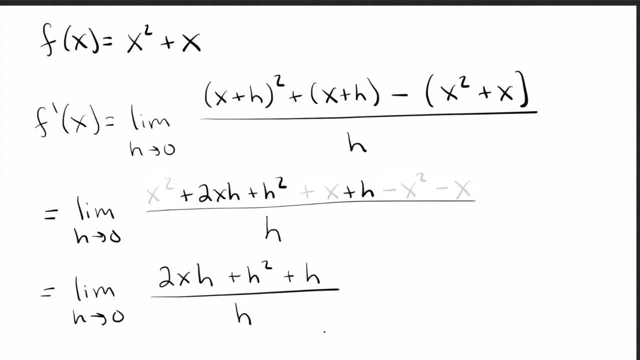 So this is good because- remember, the goal is always to plug in: h equals 0. But if I just tried to do that right now, I would be dividing by 0. I'd have a 0 on the bottom, But now I see everything has h. 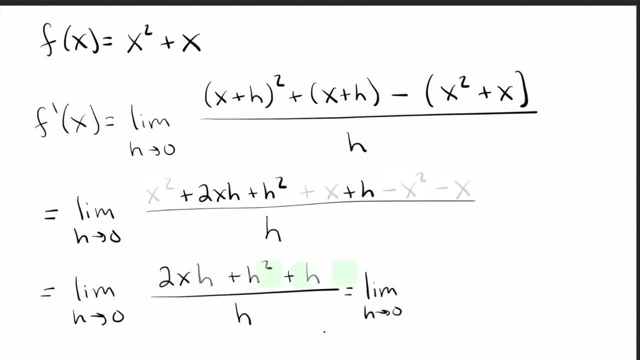 I'm going to go ahead and put the h's in it. So I like to be very careful in my work. I'm going to go ahead and factor out the h on top. So if I do that, that's what I have on top. 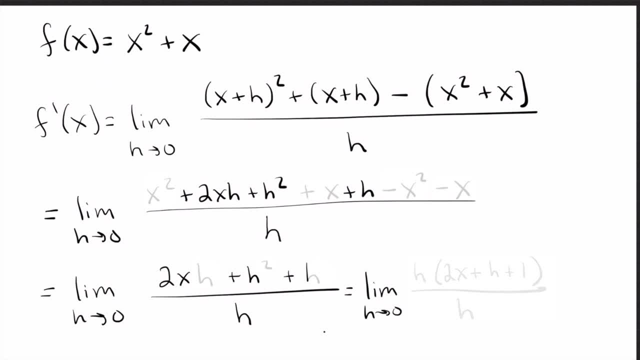 And then I can cancel out my h's. So if we go ahead and do that, we see what we end up with is the limit, as h goes to 0, of 2x plus h plus 1.. And now we can just plug in: h equals 0.. 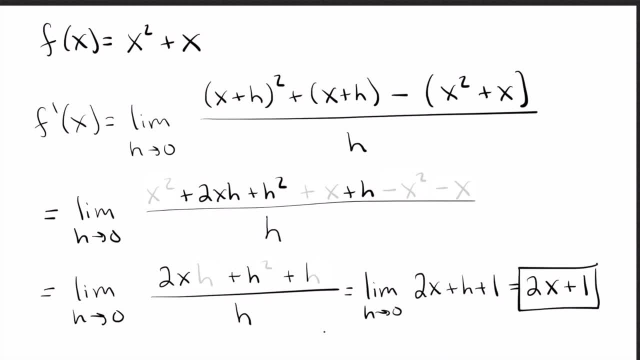 So we do that And that gets 2x plus 0 plus 1. one. So there we go. So the derivative of x squared plus x is 2x plus one. So that's a trick. you see a lot when taking derivatives using the limit definition of a derivative. is you've got. 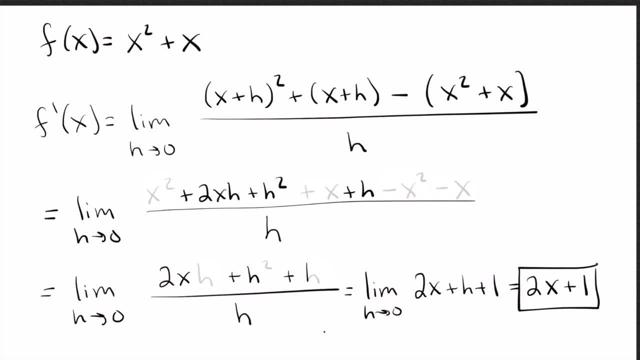 something you can square out, and if you square it, you'll end up being able to cancel lots and lots of terms and things will look much nicer afterward. So that's definitely something to keep in mind. In fact, I would say that is one of the two main tricks that shows up for taking these. 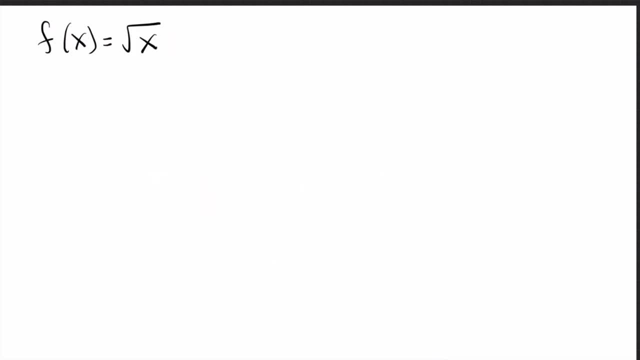 derivatives. Okay, so let's go ahead and do number four. So number four is the square root of x, and this is one that looks pretty simple, but it can really give you trouble. I mean, we'll see exactly how you can deal with that, though, So let's just jump right into the limit. definition. 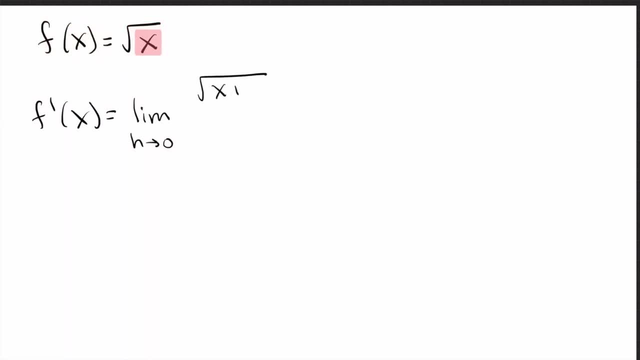 So we know. I first take my equation, I plug in x plus h minus f of x over h. Now a lot of people get here and they're just stuck because they look and they say, what the heck can I possibly do? I can't subtract those square roots, I can't cancel anything, I can't square anything out. I. 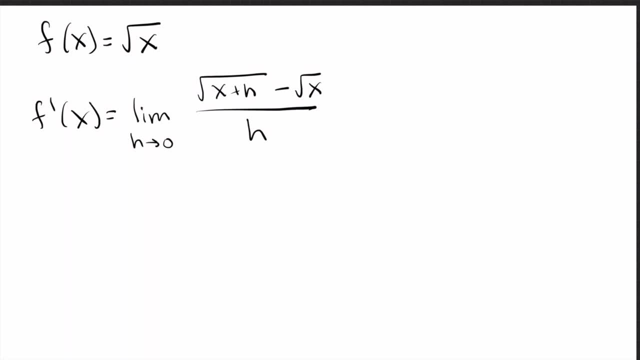 don't know where to go from here. So this is the second big trick that shows up a lot with taking these sorts of derivatives. So the trick is, what you want to do is you want to multiply the top and bottom by the conjugate of the top. Remember, the conjugate is just a fancy way of saying. 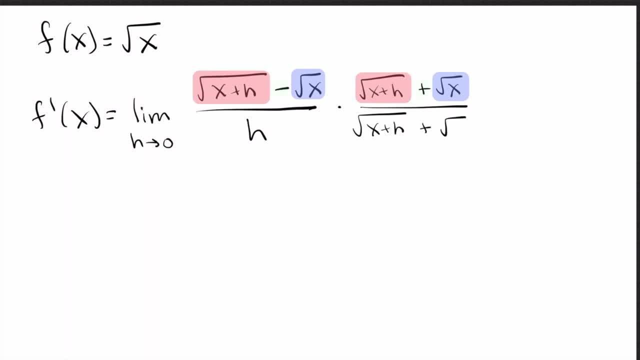 take the thing you've got on top and switch the sign in the middle, So we've got a minus in the middle. I switch it to plus h, minus h. I take the thing you've got on top and switch the sign in the middle, So that should be a plus. but everything else stays the same. And the reason we want to do. 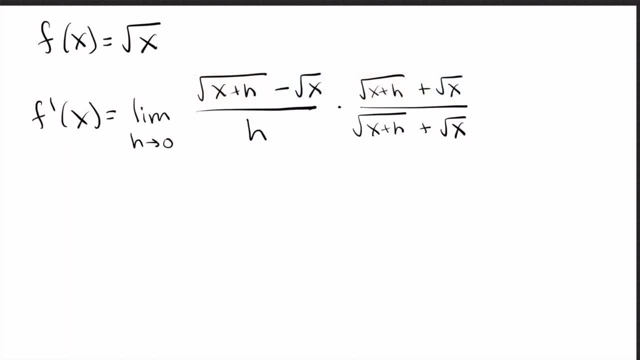 that is, it makes the top turn out much nicer. So let's go ahead and just multiply it out. So if you multiply out the top, you FOIL out the top. what we get is the first two multiply together and we get root x plus h, times, root x plus h, which is just x plus h. So that's the. 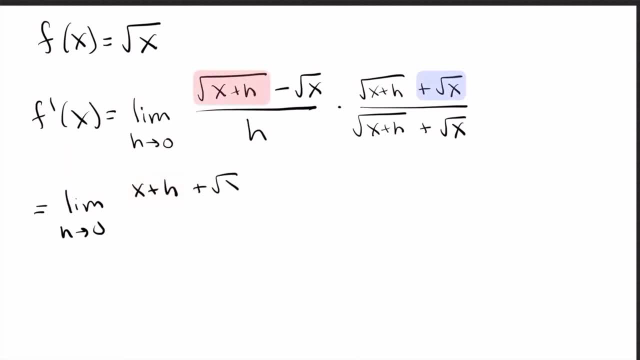 first term. Then in the middle we get a plus root x times root x plus h. And then the next term in the FOILing gives us the opposite of that, And this is really the power of multiplying by the conjugates. You get these two terms in the middle which are going to cancel. 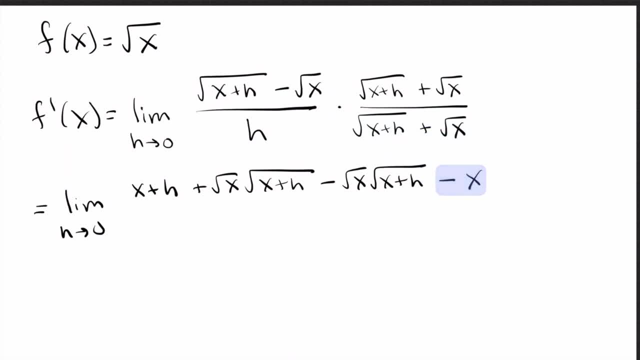 And now we get root x times root x, which is just x On the bottom. actually, what I'm going to do is I'm not going to multiply it out at all, And if you were the one doing this, you might not know. 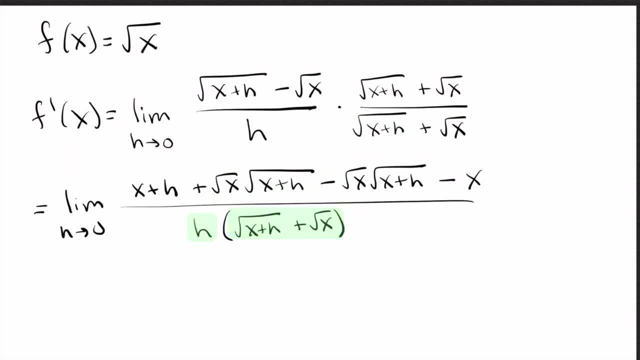 that you shouldn't multiply it out. I mean, it's not going to hurt you to multiply it out, but it'll save you time if you don't. So let's go to the next step. here We'll see why we're doing this the way we are. 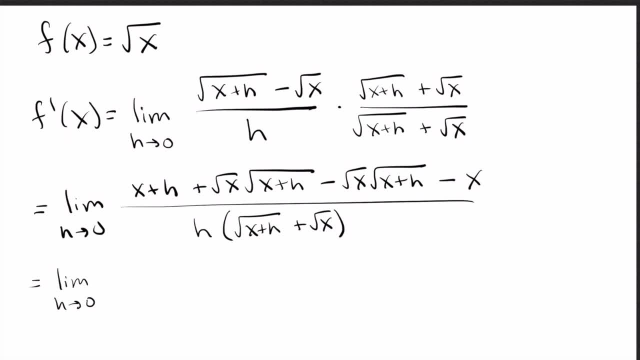 So on top, let's see what we get that cancels out. So I have an x that cancels out, with a minus x at the back. That's great. I have an h on top And now I have root x times: root x plus h. 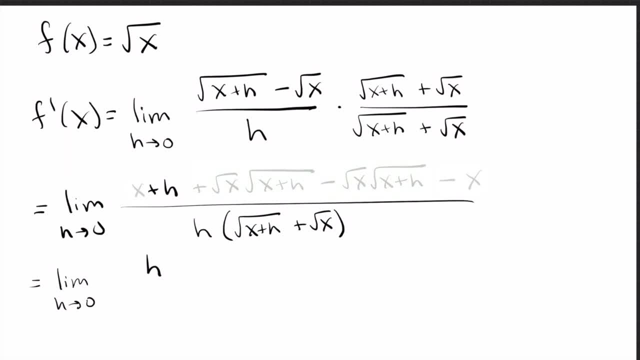 which cancels with minus root x times root x plus h. So that's it. There's just h on the top, Right And the bottom. now you can kind of see why I did not want to multiply that h on the bottom, because I was going to cancel it at the next step. So if I would have multiplied it in 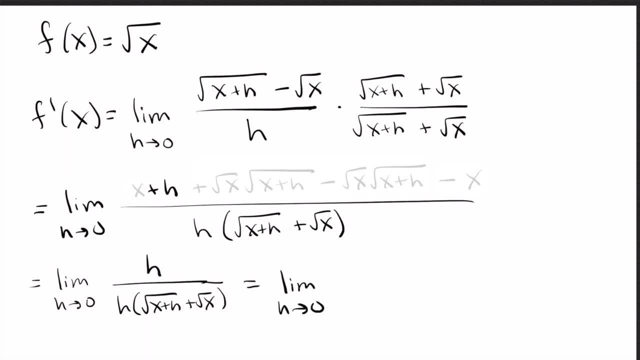 I would have had to factor it back out, So I'll cancel those h's. I'm left with 1 over root x plus h plus root x, And now I can plug in: h equals 0. And if I do that I get root 1 over x plus 0. 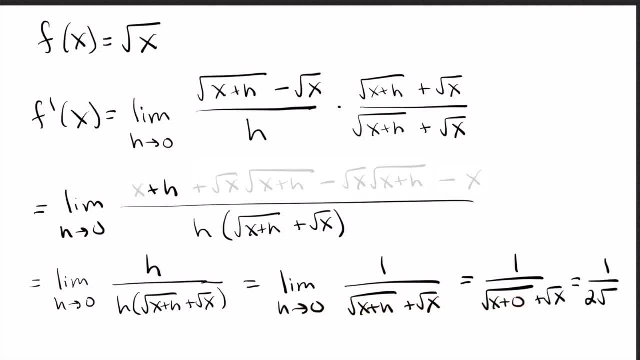 plus 1 over root x. That's just 1 over 2 root x. And there we go. We have taken the derivative of the square root of x. So we see that actually this one maybe looks bad at first, But once you do. 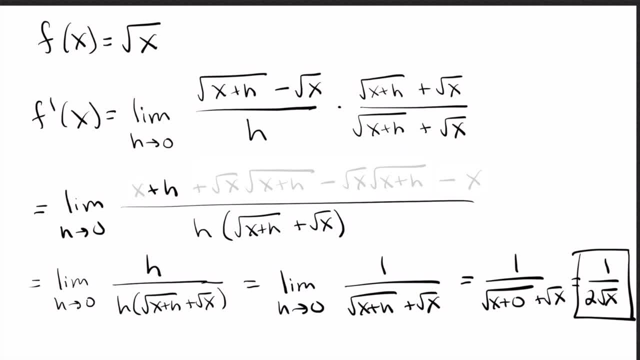 the multiplying. it's actually pretty short. In fact, if you did problem 3 with me, you see this is actually less work than problem 3.. OK, so with that let's go on and do problem 5.. So let's go. 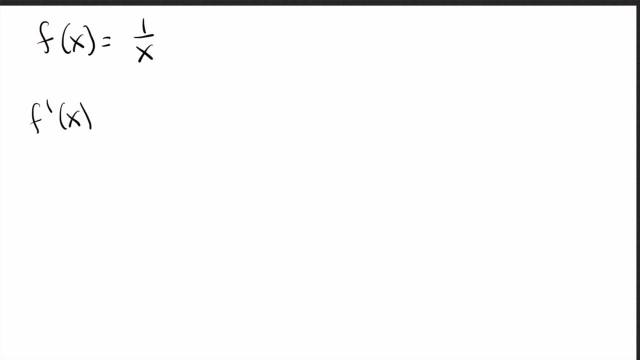 ahead and start working through this one. So this one really is the third and final trick that you see a lot when working with these derivatives. So the first trick came from problem number 3, where, if you can square something out, oftentimes it is helpful to do so. The second trick is multiplying the top. 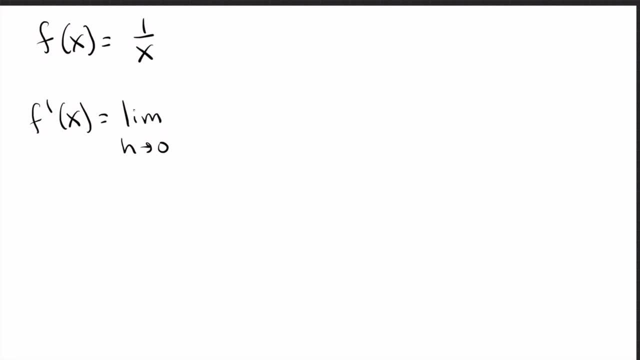 and bottom by the conjugate, like we did in problem number 4.. So here's our final trick. So let's go ahead and get started. So I plug in x plus h minus f of x over h. So again, when you get here it may not be obvious what you should do next, And that's why I say this. 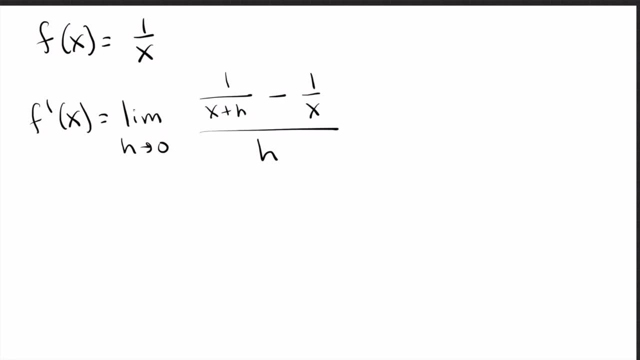 is sort of another trick that shows up, But really all you do is you have fractions and you're subtracting them. Well, if you have fractions and you're subtracting them, how about you subtract them? right, Get common denominators and subtract them. So let's go ahead and do that. 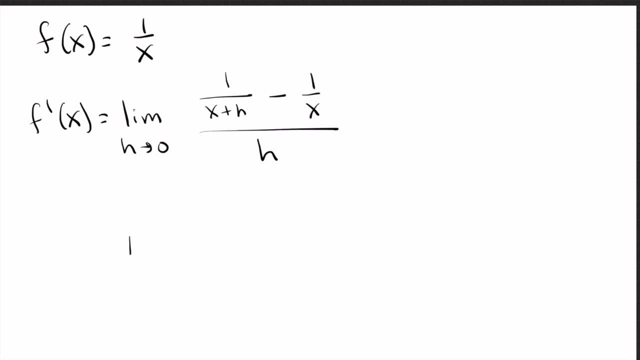 I'll do my scratch work off to the side here. So if I have 1 over x plus h minus 1 over x, my common denominator is going to be x times x plus h. So this one I multiply top and bottom by x plus h, This one top and bottom by x. And if I do that what I get is x over. 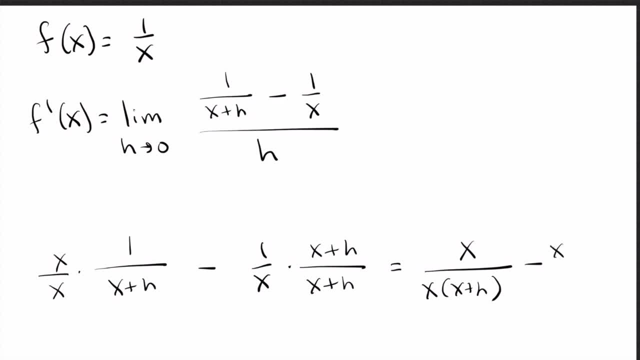 x times x plus h minus x plus h over x times x plus h. Okay, On the top, the x minus x cancels. I'm left with minus h over x times x plus h. It's a little messy but no big deal. 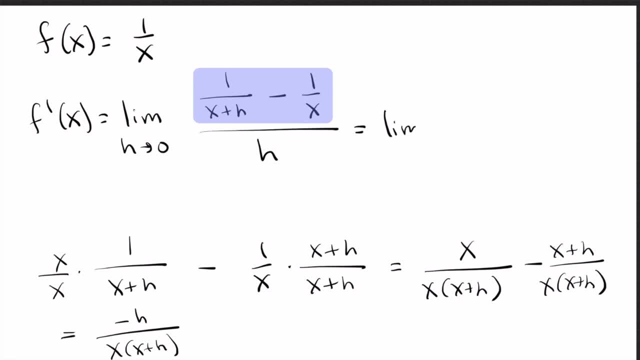 Okay, So let's go ahead and put that in on the top, So I'll keep my limit. And then we just saw that the top can be rewritten as negative h over x plus h, So I'm going to put that in on the top. 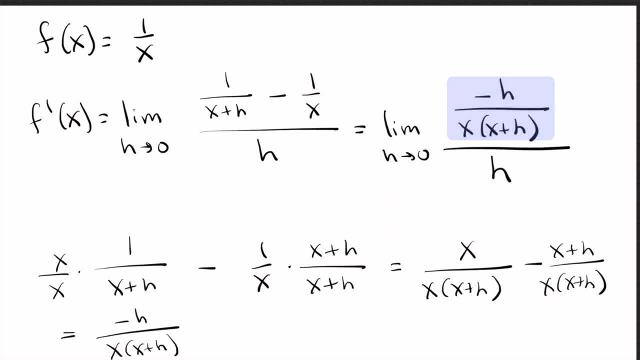 x times x plus h, that whole thing over h. Okay, Let's keep going. So the next step is just to clean this up a little bit, And what I want to do is just not have this double fraction. So dividing by h is the same thing as multiplying by 1 over h, So I keep the top of the fraction.